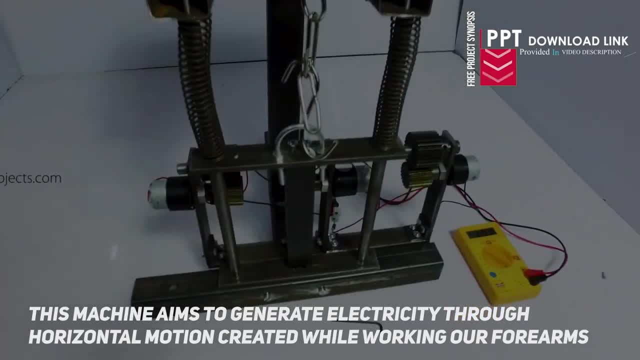 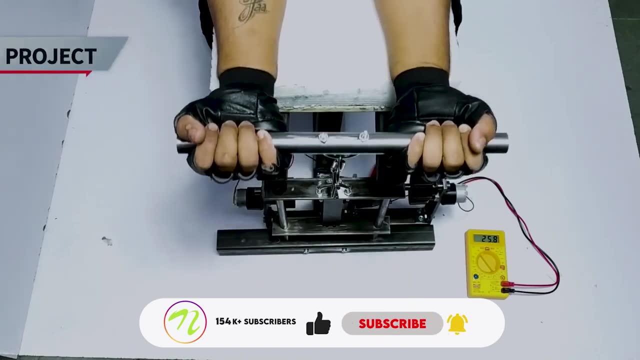 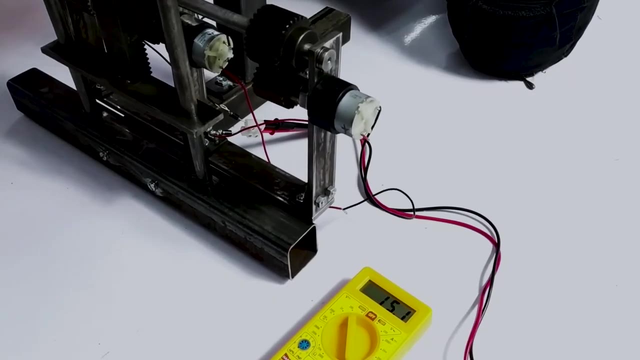 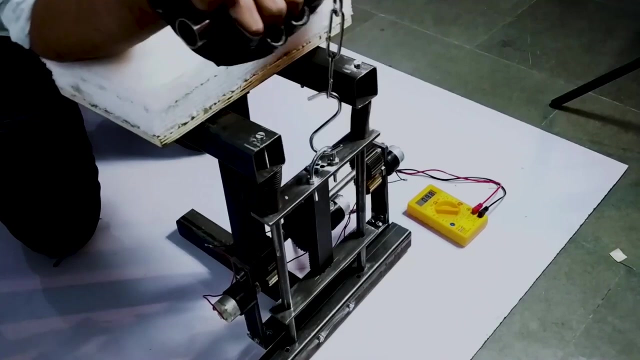 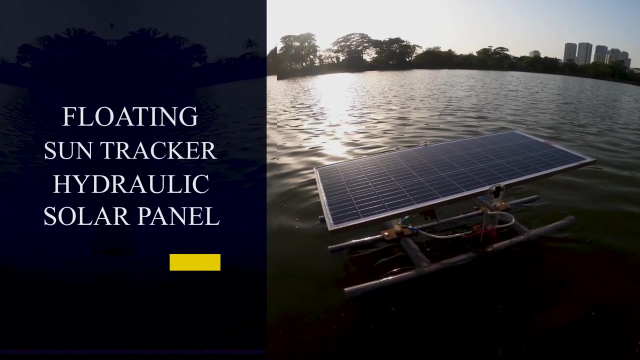 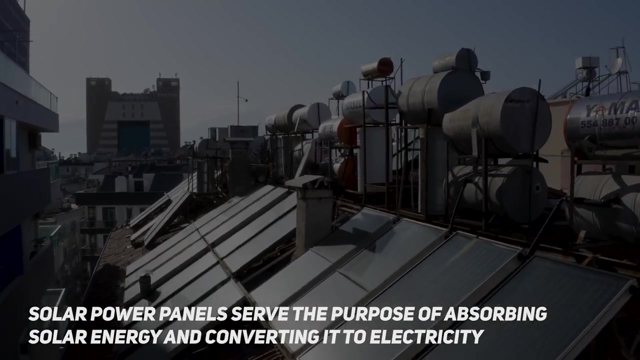 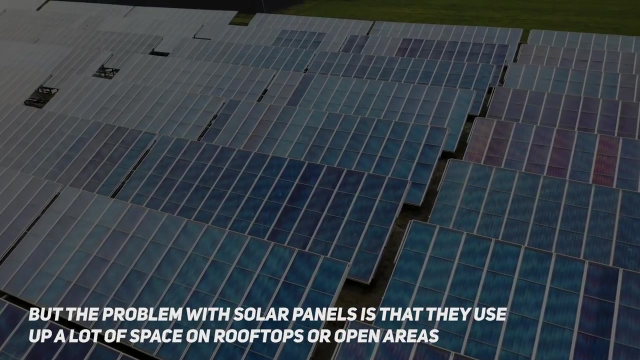 generate electricity through horizontal motion created while working our forearms. Floating Sun Tracker. Hydraulic Solar Panel. Solar power panels serve the purpose of absorbing solar energy and converting it to electricity, But the problem with solar panels is that they use up a lot of space on rooftops or open areas. 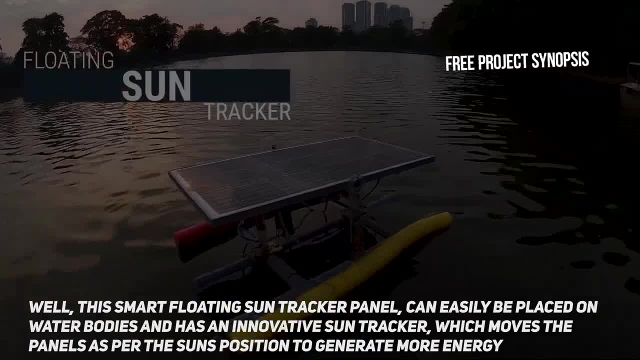 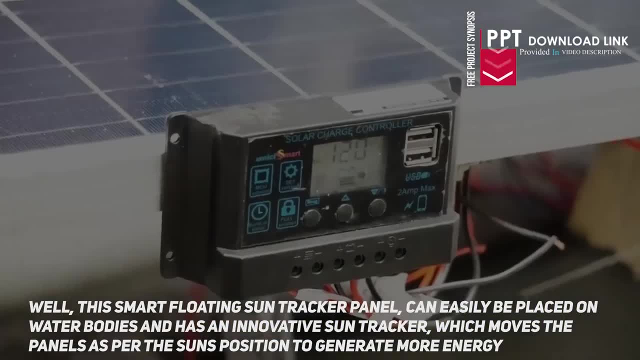 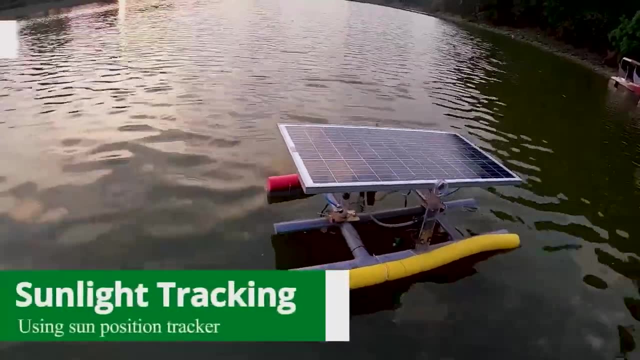 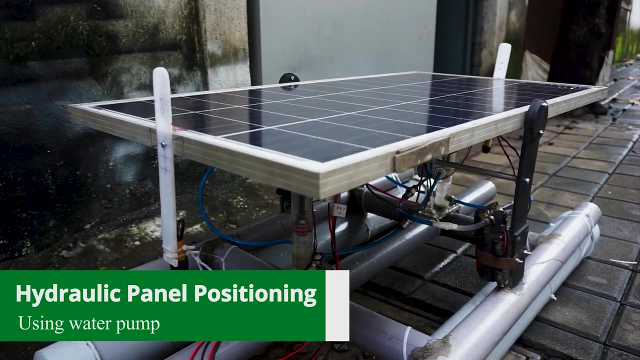 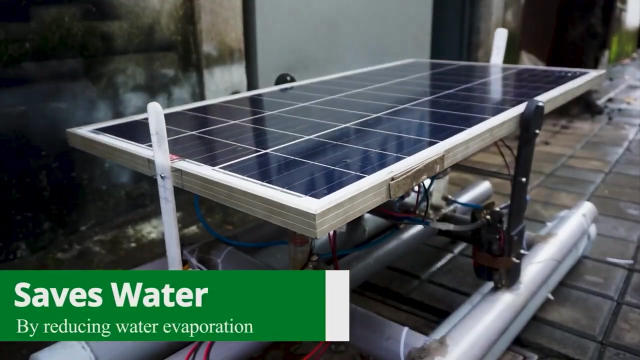 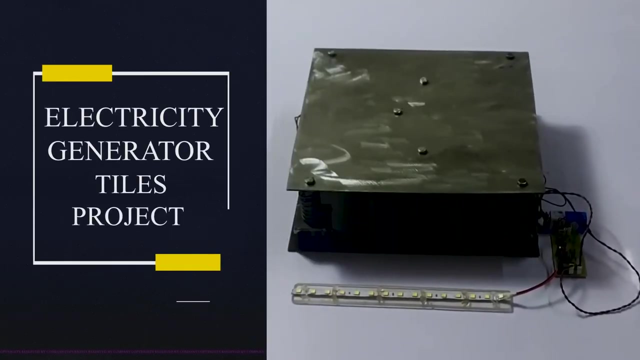 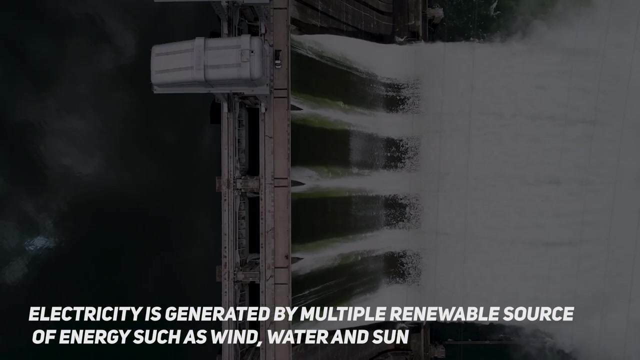 Well, this smart floating solar tracker panel can easily be placed on water bodies and has an innovative sun tracker which moves the panels as per the sun's position to generate electricity. To generate more energy, Electricity Generator Tiles Project. Electricity is generated through multiple renewable sources of energy, such as wind, water and sun. 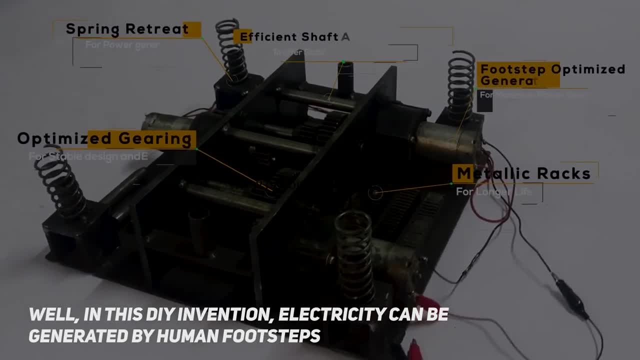 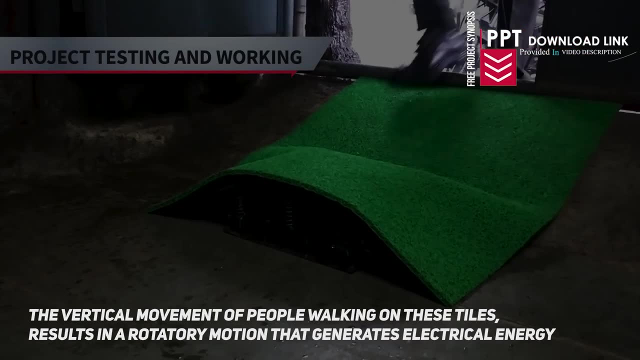 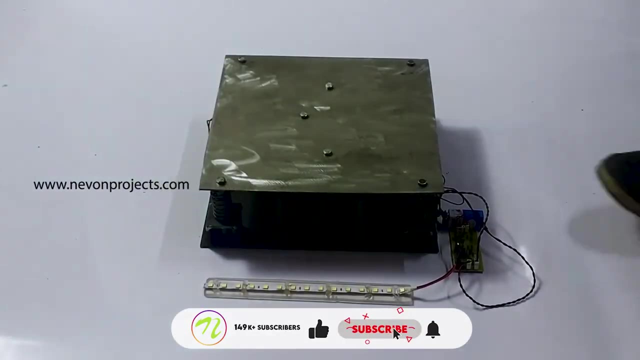 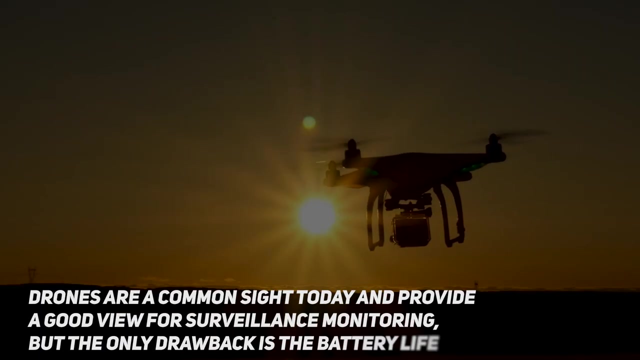 Well, in this DIY invention, electricity can be generated by human footsteps. The vertical movement of people walking on these tiles results in a rotatory motion that generates electrical energy. Self-Charging Solar Power Drone Drones are a common sight today and provide a good view for surveillance monitoring. 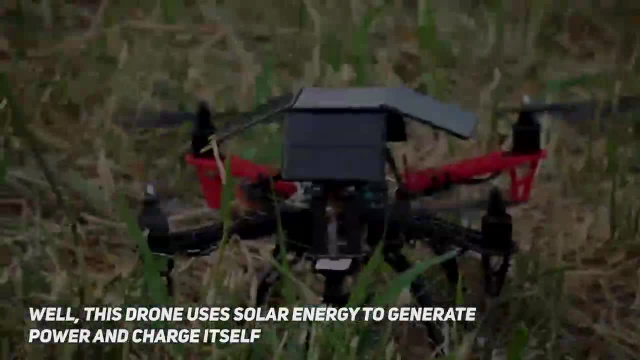 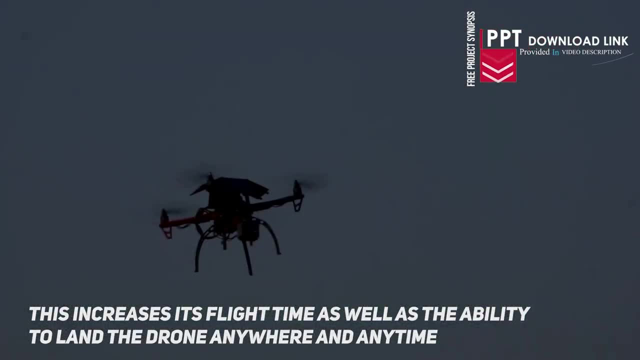 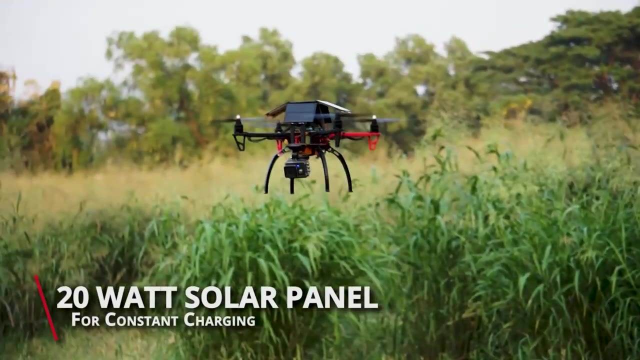 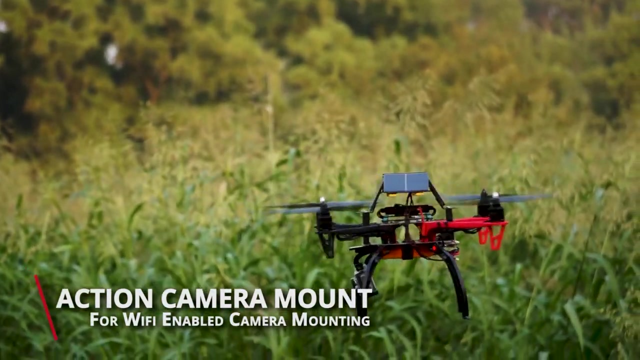 But the only drawback is the battery life. Well, this drone uses solar energy to generate power and charge itself. This increases its flight time. as well as the ability to land the drone anywhere and anytime, It's also a great way to store energy.